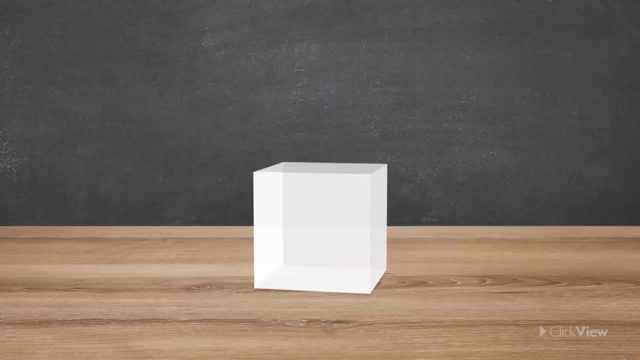 No, not that type of face. The edge of a 3D shape is the line where two of its surfaces meet, And the corner is where two or more edges meet. A corner can also be called a vertex. The faces of 3D shapes often contain 2D shapes that you may already know. 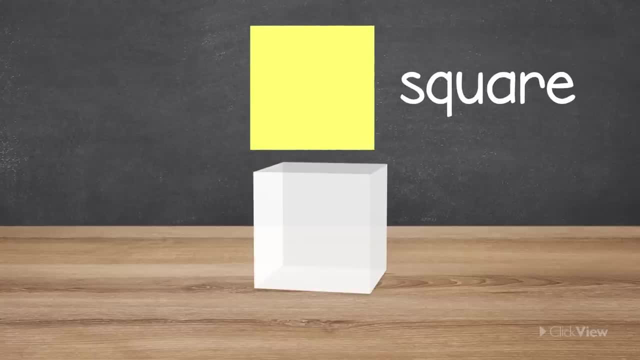 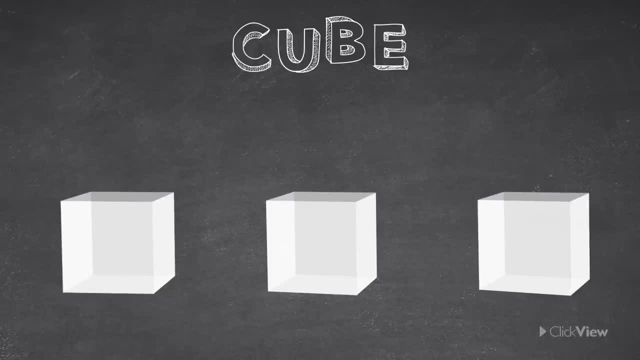 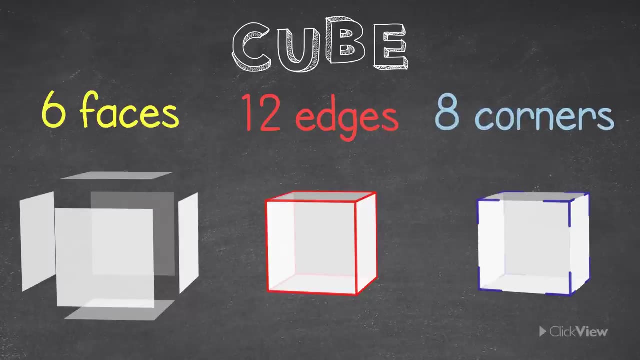 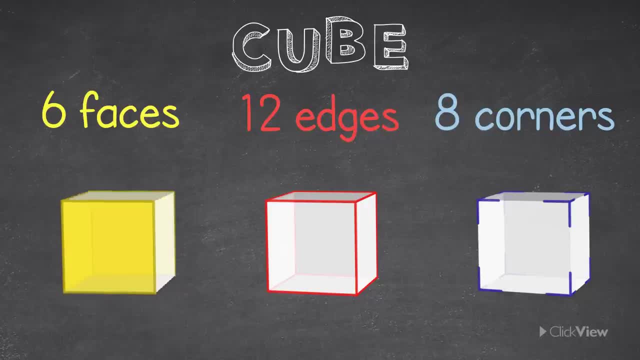 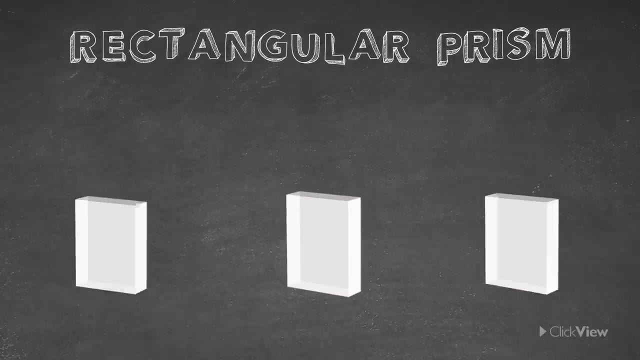 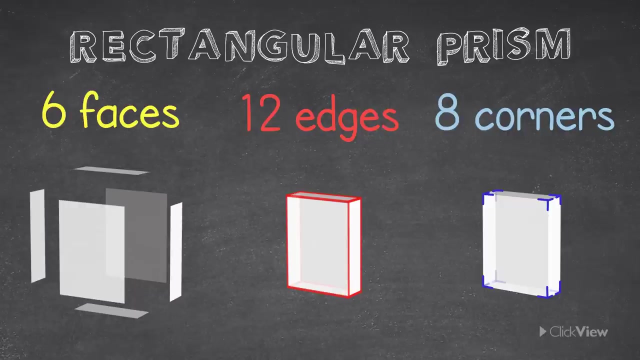 Can you see how each face of the cube is a square? Yes, that's right. a cube has 7 faces and 6 corners. This shape is called a rectangular prism. A rectangular prism has 6 faces, 12 edges and 8 corners. 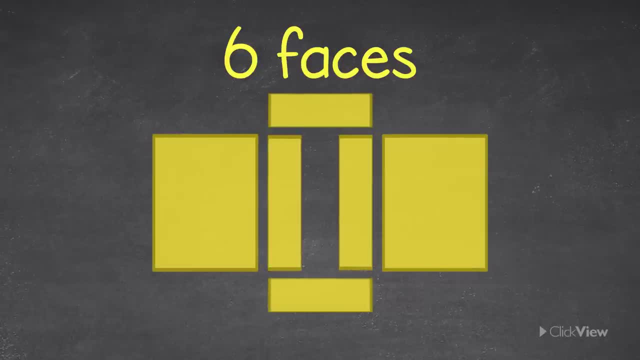 It's very similar to the cube, except instead of all the faces being squares, they are rectangles. The opposite faces of the rectangular prism are always the same size. We registered them as 4лож fashion, which means they are the cut off volume and tied to the dividing chain of created types. 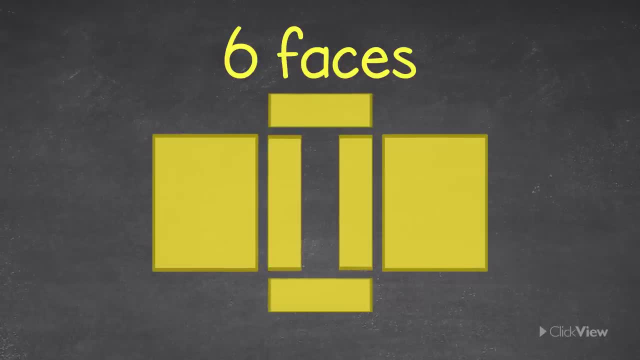 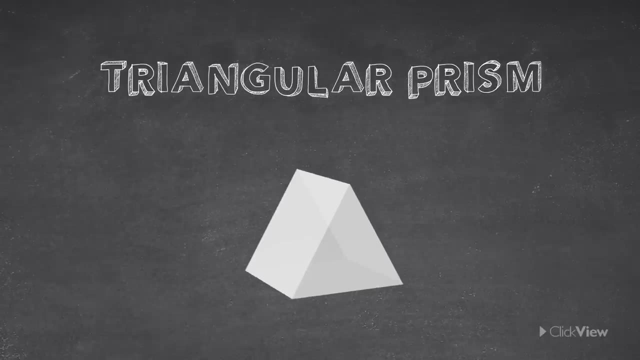 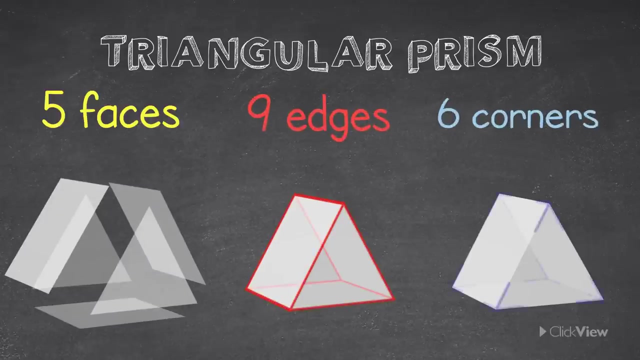 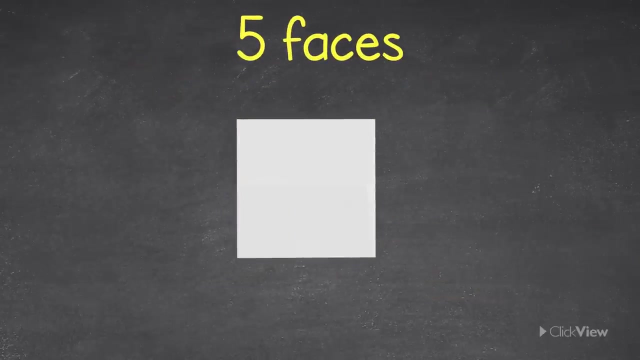 The 3 Rhombs logo is the chrononut model. We registered them in July, August and in November. This shape is a triangular prism. A triangular prism has five faces, nine edges and six corners. Triangular prisms have two faces that are triangles and three. 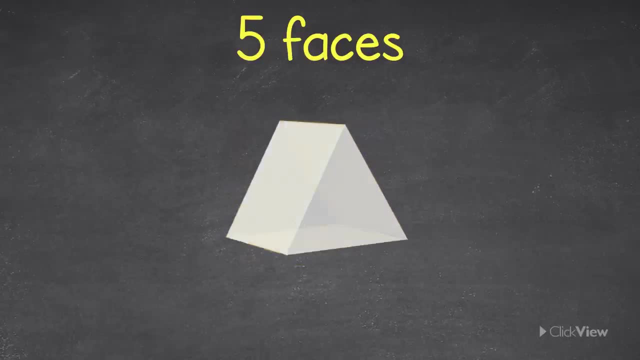 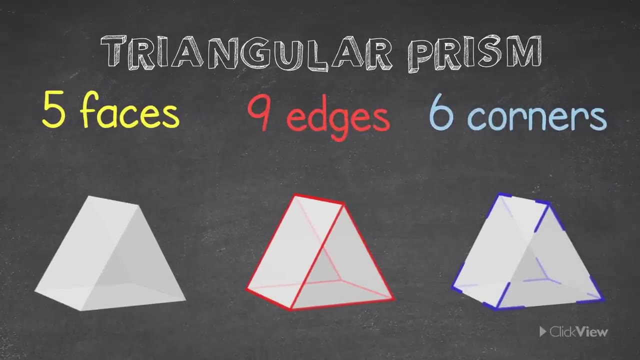 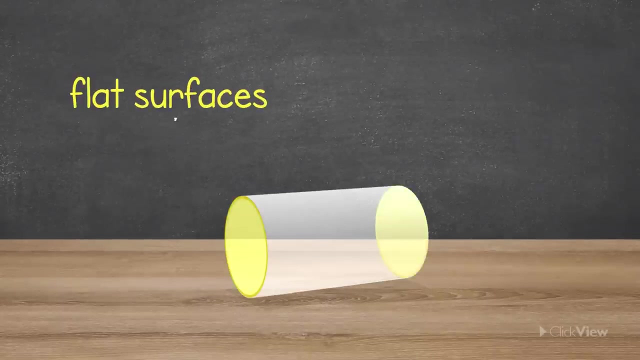 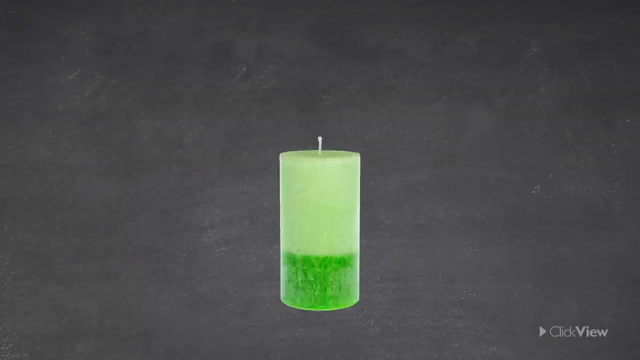 faces that are rectangles. The two triangle faces are always the same size. However, some 3D shapes have more than just flat surfaces. Some have curved surfaces, but we don't call them faces, because faces are always flat. This shape is called a cylinder. A cylinder has two circles on each end that are the same size. 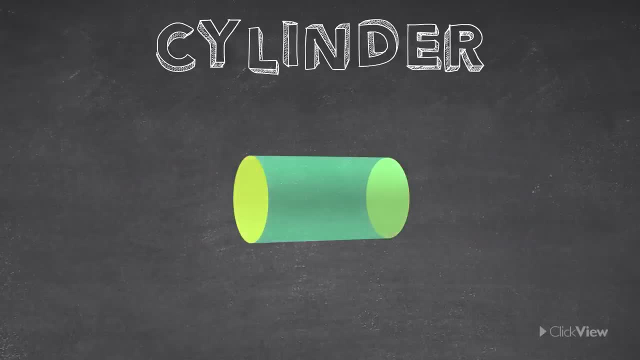 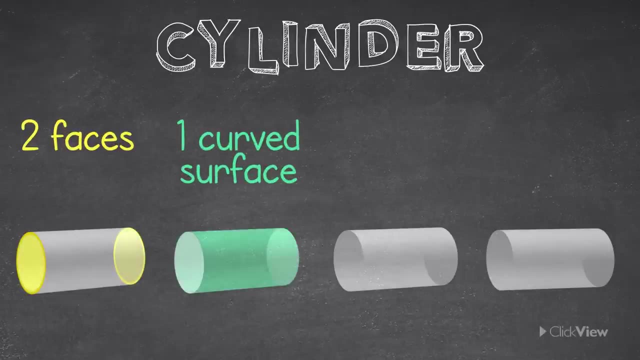 with a tube in the middle. It has two flat faces and one curved surface. The cylinder also has two edges but no corners. Remember, a curved cylinder has two edges but no corners. Remember, a curved cylinder has two edges but no corners. 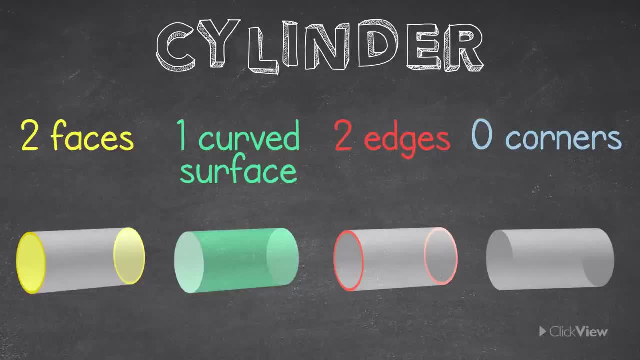 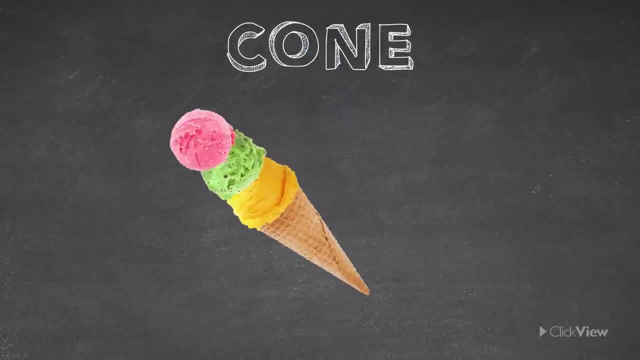 Remember, a curved cylinder has two edges but no corners. A corner is where two or more edges meet. In a cylinder, there are no corners because its two edges do not meet. This is a cone, Not an ice cream cone, unfortunately, but it is the same shape. 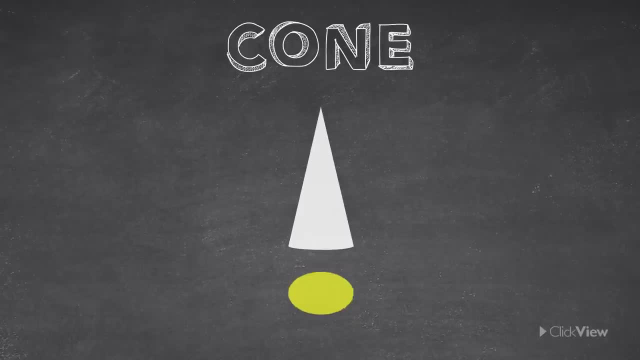 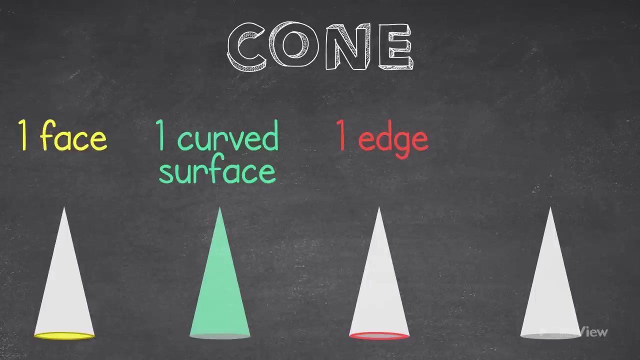 A cone has a circle at its base and a point at the other end. A cone has a circle at its base and a point at the other end. It has one flat face, one curved surface, one edge around its base, but no corners. 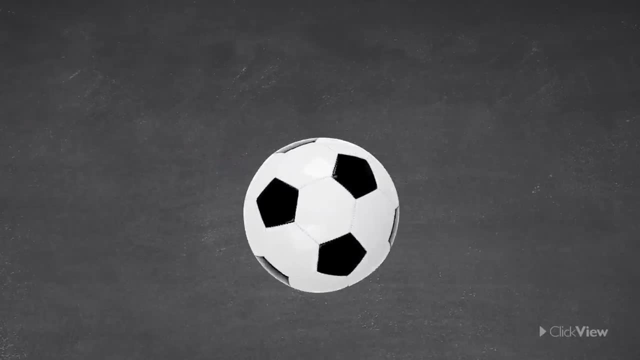 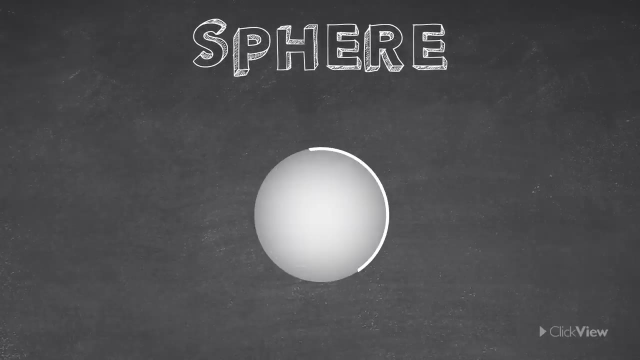 It has one flat face, one curved surface, one edge around its base, but no corners. This unique shape is a sphere. It's perfectly round, just like a ball. This means it has no flat faces, no edges and no corners. 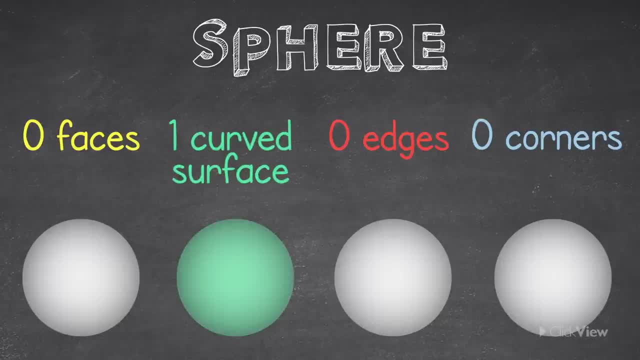 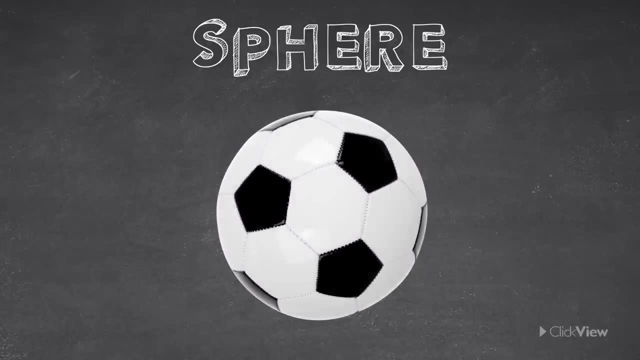 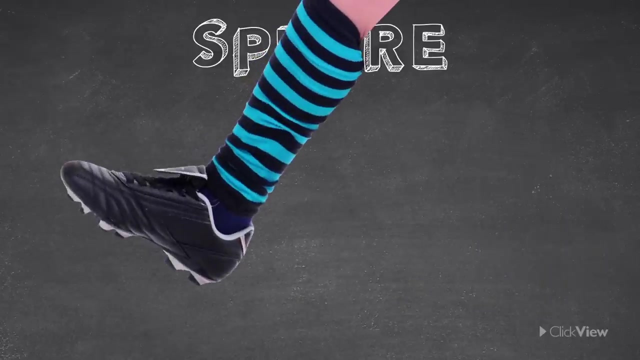 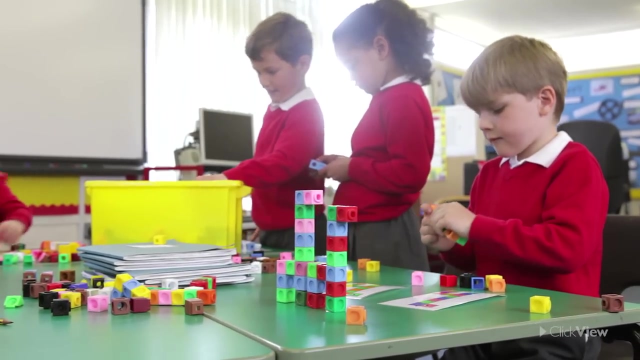 Just one curved surface. How unique is that? That's what makes a sphere the perfect shape for a ball. It rolls around easily in any direction and you can kick it without banging your toe on a sharp corner. Now that you know some three-dimensional shapes, perhaps you can spot a few examples of 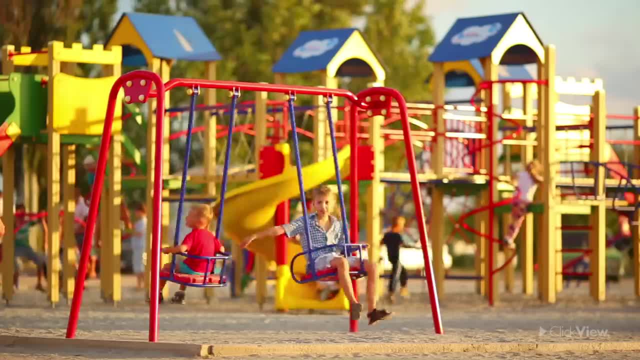 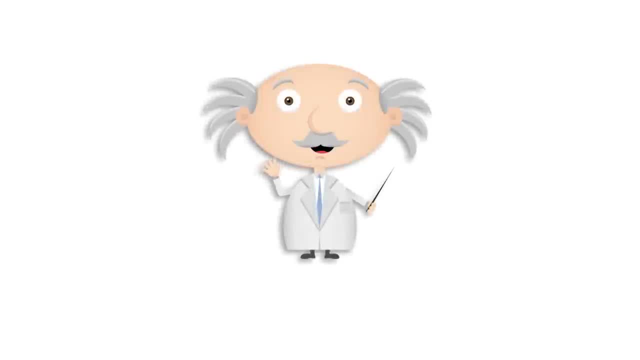 them in your classroom or out in the world. Now that you know some three-dimensional shapes, perhaps you can spot a few examples of them in your classroom or out in the world. Find them outside in the playground. Hee-hoo, Hee-hee.